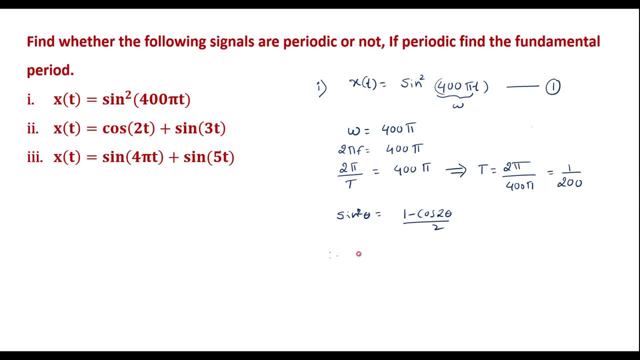 Therefore, I can represent it as x of t is equal to one minus cos two. two into 400, that is 800 pi t divided by two. or I can represent it as x of t is equal to one by two minus one by two, cos 800 pi into t. 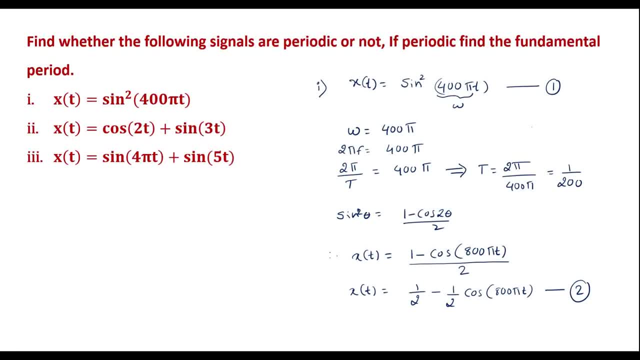 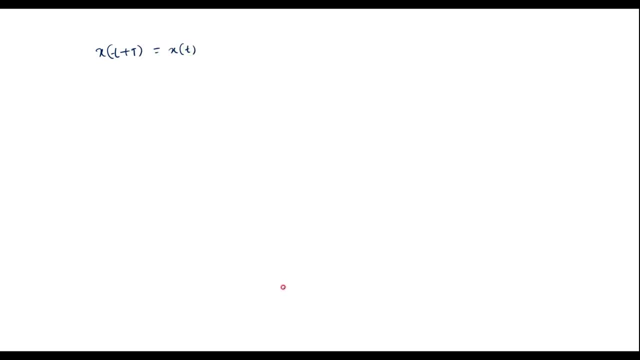 Call it as equation two. Now we know that signal is said to be periodic if x of t plus t is equal to x of t. now I will try to represent equation two as x of t plus t. Therefore I can write x of. 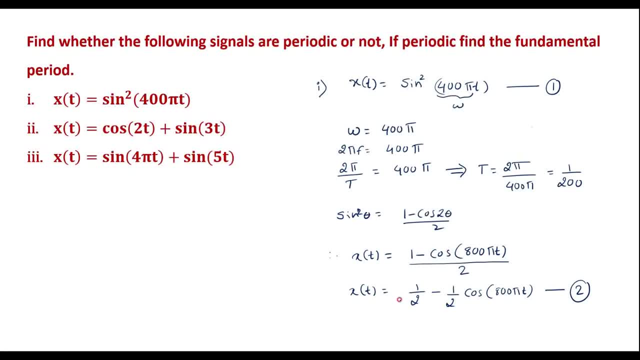 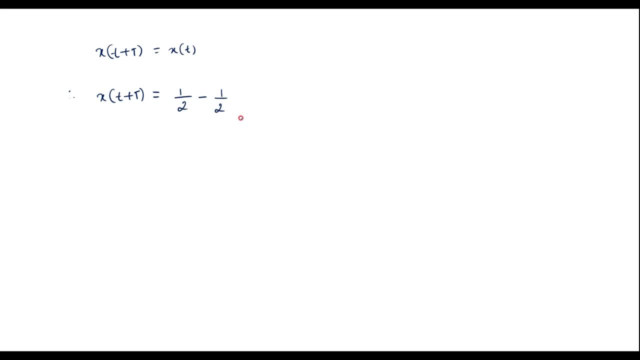 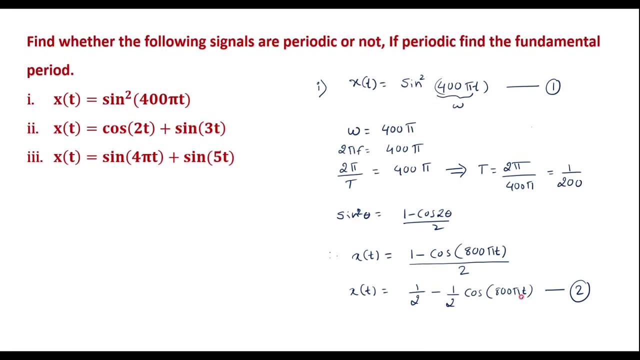 t plus t is equal to. so replace t by t plus t in this equation So that I can get it as 1 by 2 minus 1 by 2. we have cos 800 pi plus 800 pi into t, that is, t is nothing. 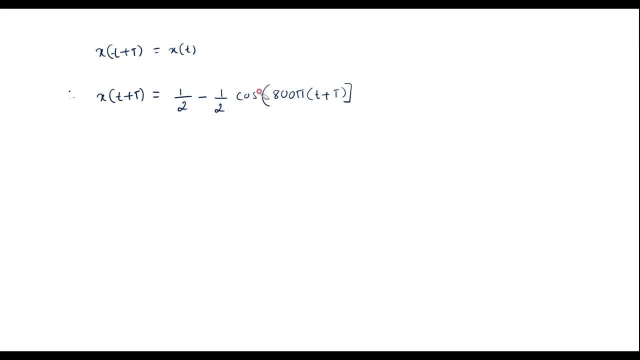 but t plus t, or I can represent it as 1 over 2 minus 1 by 2, cos 800 pi. t plus 800 pi into t, or I can simplify this as 1 by 2 minus 1 by 2, cos we have 800 pi t. 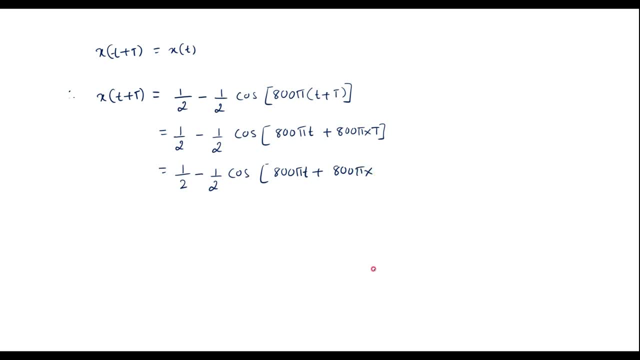 plus 800 pi into. so already we have calculated t and its value is 1 over 200, that is, 1 by 200, or I can simplify this as 1 minus 1 by 2 minus 1 by 2 cos, we have 800 pi t plus. here we have. 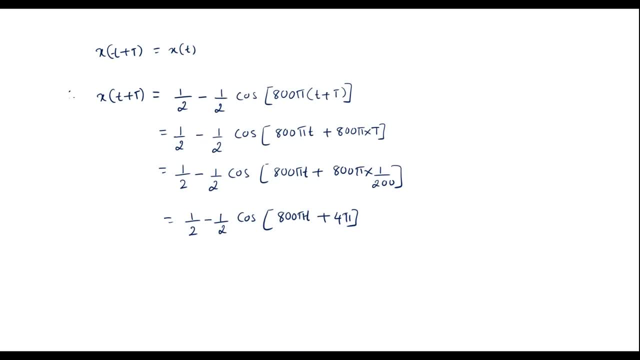 4 pi. so we know that cos a plus b can be represented 2. so we know that cos a plus b can be represented 2. so we know that cos a plus b can be represented as cos a, cos b minus sin a, sin b. So in this case a value is 800 pi, t and b is nothing but. 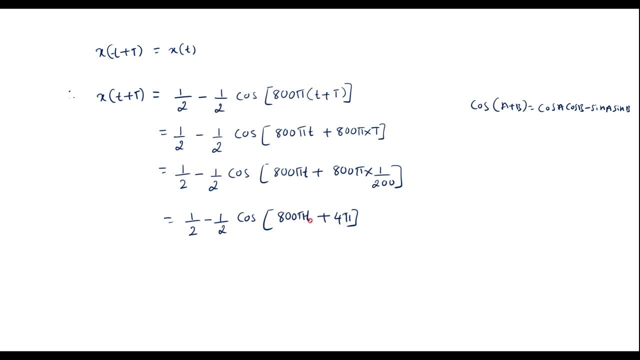 cos 4 pi, So cos 800 pi t, plus into cos 4 pi, So cos 4 pi is 1 and sin 4 pi is 0. So that I can represent it as 1 by 2 minus 1 by 2 cos. that is cos a into cos b. Here cos a is: 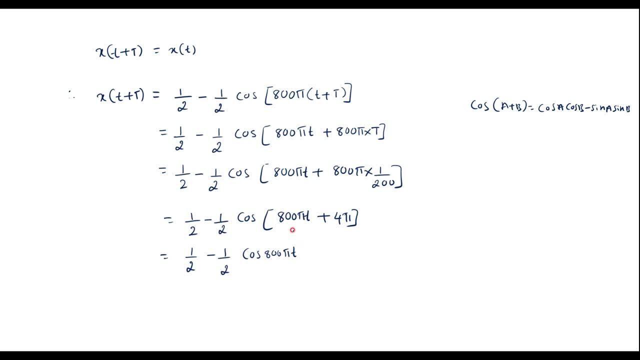 800 pi. t cos b, cos 4 pi is 1 and sin term will be 0. So x of t plus t will be equal to this one, which is nothing but x of t. So we got x of t is equal to x of t plus t. Therefore. 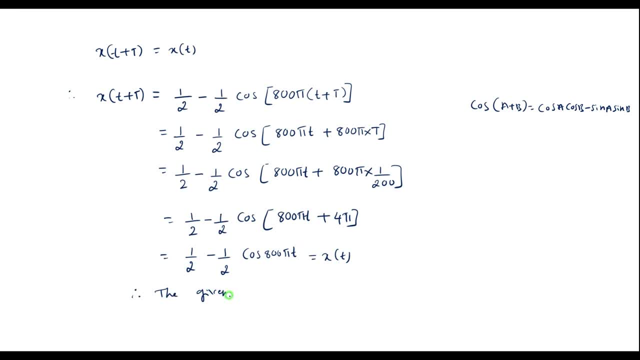 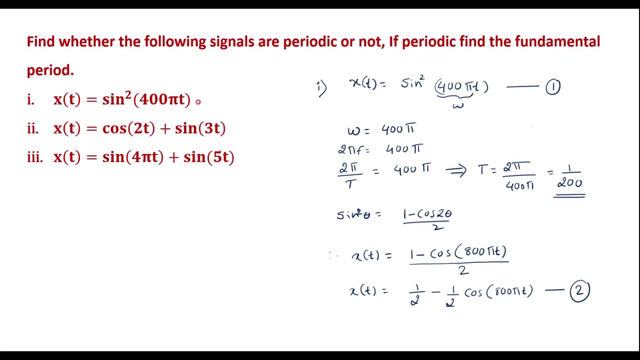 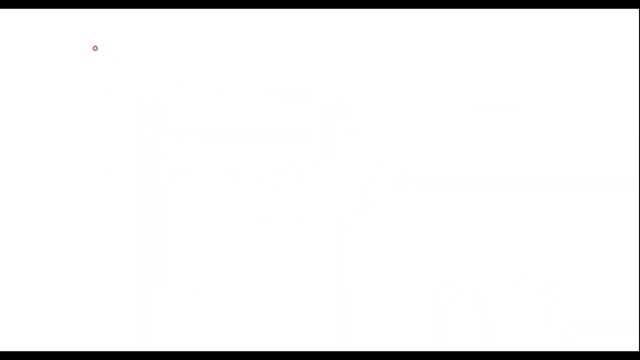 the given signal is periodic. So given signal is periodic. with period, t is equal to 1 upon 200.. Let me consider the second signal that is: x of t is equal to cos 2 t plus sin 3 t. So this is the composite signal that is x of t. is consists of two different signals. 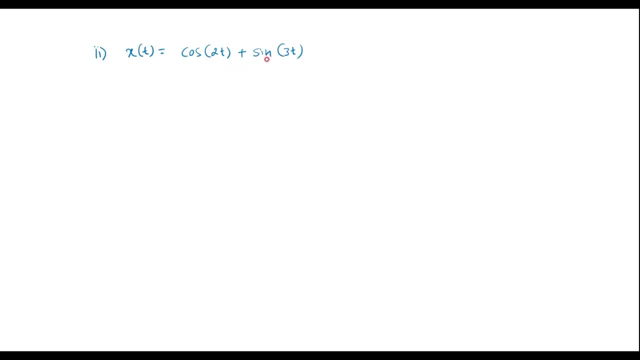 One is cos 2 t signal is added with other signal node as sin 3 t. Now we will see how to find the fundamental periodicity for composite signal. So here we can see that it is of form cos omega t. So I can say omega 1 is equal to 2.. Here omega 2 is equal to 3. So we know that. 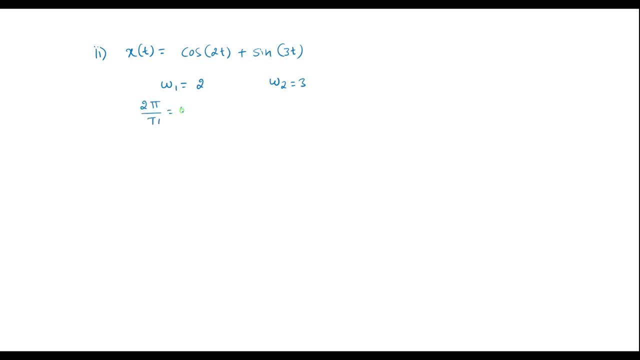 omega 1 is nothing but 2, pi by t1 is equal to 2.. Here we have 2. pi by t2 is equal to 3.. Or here, t1 is equal to 2, pi by 2, which is nothing but 2, pi by t2 is equal to 3.. So here we have 2. pi by t2 is. 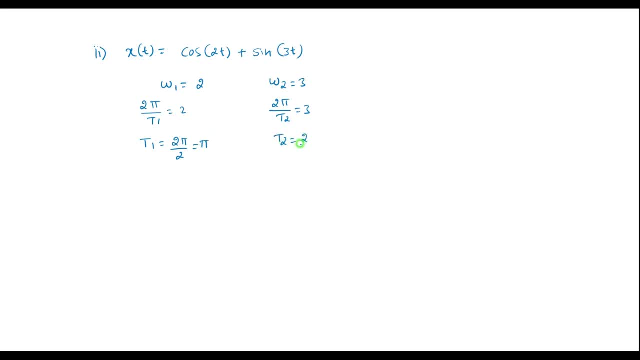 pi. and here we have: t2 is equal to 2 by 3 pi. So now the next step is: we have to perform t1 by t2.. That is t1 by t2.. t1 is pi, t2 is 2 pi by 3 pi. 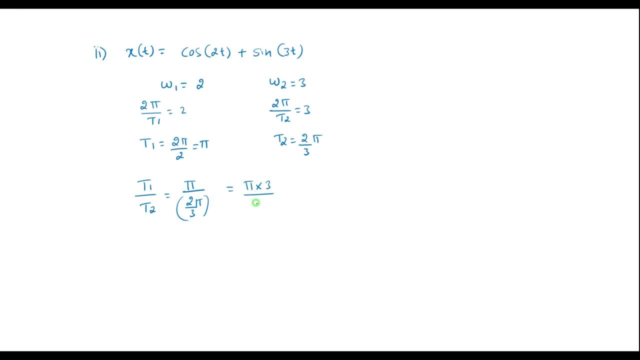 That is nothing but pi into 3 divided by pi by t, Now s is 1 pi by t2 by t1 is equal to 1 pi by t2, 2 pi, which is nothing but 3 by 2.. So T1 by T2 is rational, which is rational Rational. 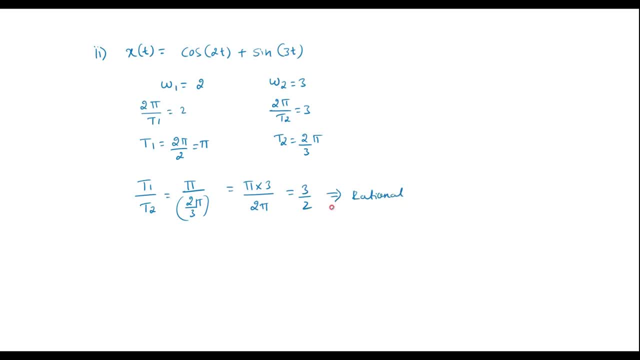 means if it is A by B form, then the signal is said to be periodic. Therefore, signal is signal X of T is periodic. So this is how we supposed to find the periodicity. if the signal is composite signal, We will see the period of this signal. 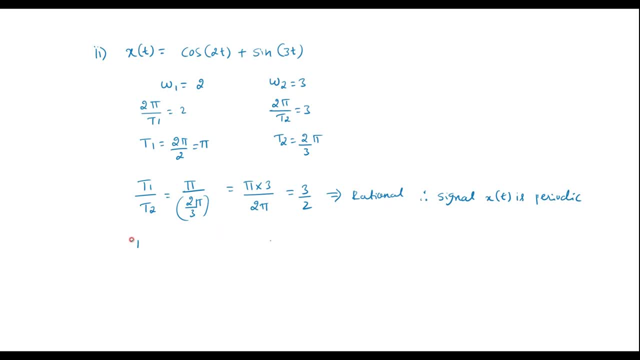 The period of the signal can be calculated using the formula. Here I will tell you the direct way of calculating the period of the signal. The period of the signal is given as by. it is calculated as, say, t0 is period of the signal, which is equal to LCM of t1 and t2.. 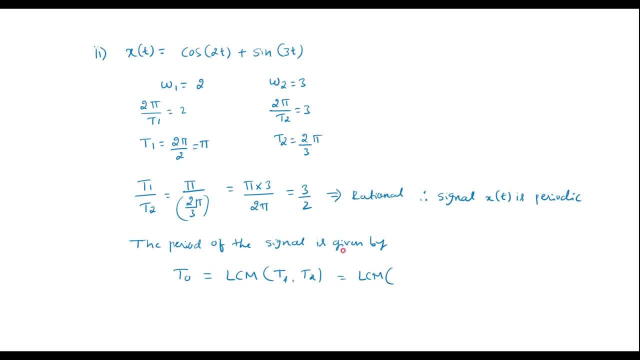 So that is nothing. but LCM of t1 is pi and t2 is 2 by 3 pi. So here pi can be represented as pi by 1.. So to find the LCM of these two terms then the direct method is: t0 is equal to, we supposed. 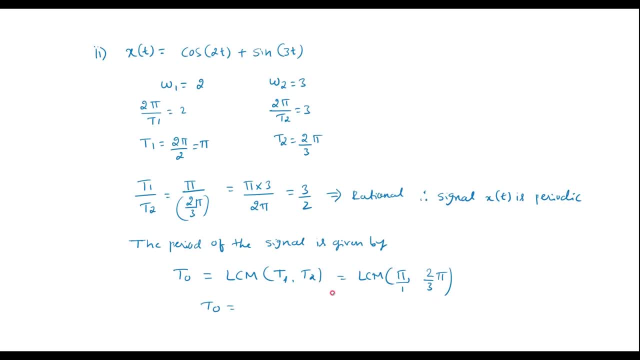 to take the LCM of numerator and HCF of denominator, that is LCM of pi, 2 pi denominator, HCF or GCD- both are same- is 1 comma 3.. So here the LCM of pi and 2 pi is 2 pi.